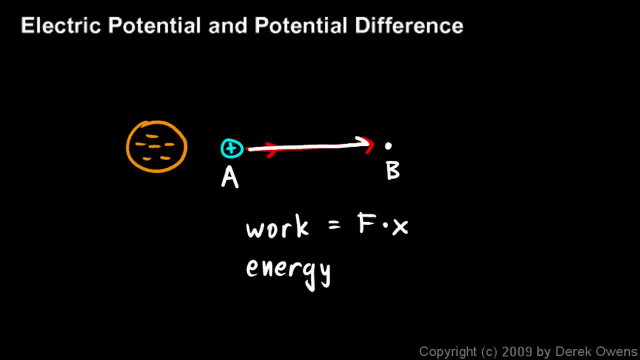 So we've expended energy. When we push this, push it over from A to B, we have expended energy. If you grab that little particle with your hand and you push it, you've expended energy. Energy has left your body. Now here's the question: Where has the energy gone? 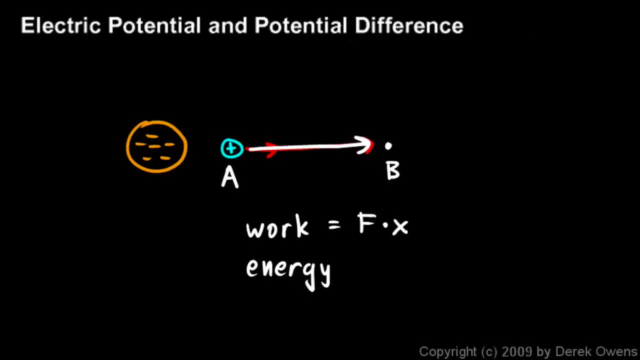 The energy that we had to expend to push that particle from A to B. where did it go? We know that it didn't simply disappear, because energy is conserved. You remember the law of conservation of energy. Energy is not created or destroyed. 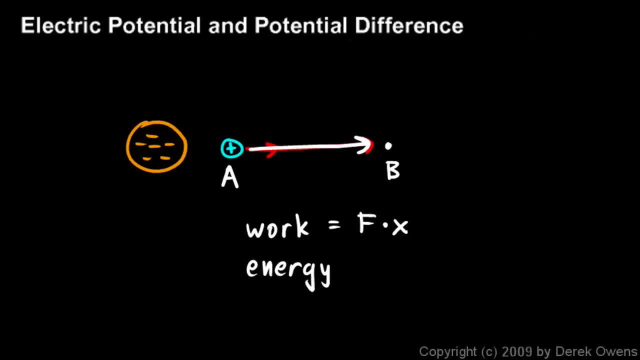 Where did the energy go, The energy that we used up pushing it from A to B? where did it go? It turns out that it has gone into potential energy, And specifically we're talking about electrical potential energy, And this is remarkably similar to gravity. 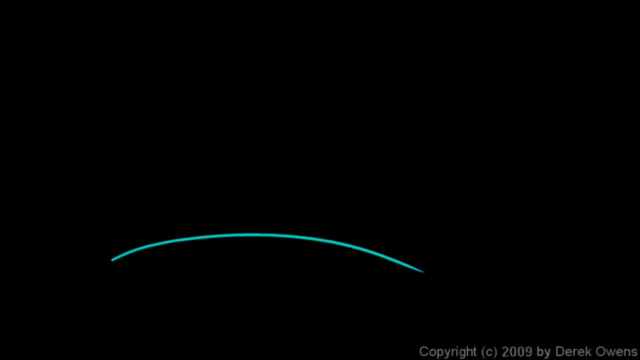 If you imagine the surface of the earth down here And here's some mass m And you want to lift the mass against the force of gravity, Then you have to exert some upward force through some distance that you're lifting it, And when you do that you expend energy. 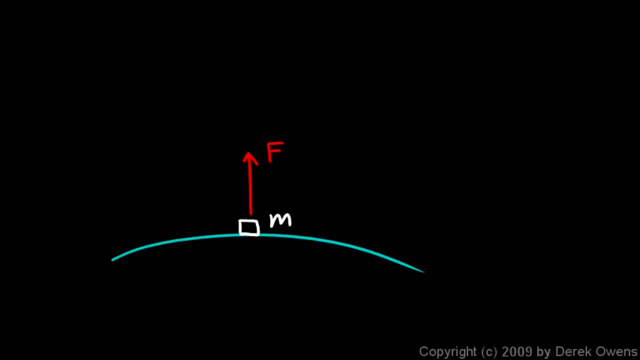 And the energy you expend goes into the mass as potential energy And specifically it's gravitational potential energy. It has potential energy because it's at a point of higher potential in the gravitational field. That same concept applies electrically When we push this particle from A to B. 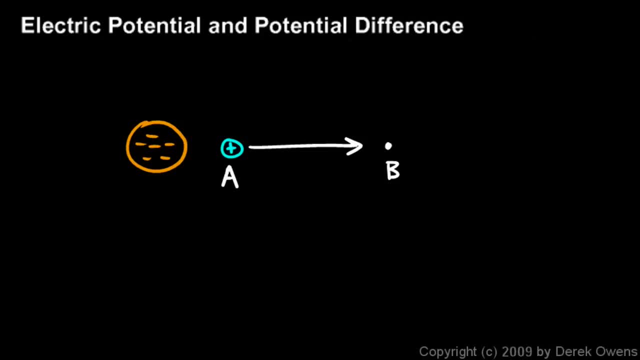 we're expending energy And that energy is going into electrical potential energy And that particle sitting here at B is at a point of higher electrical potential, A point of higher potential energy in the electric field, And that's a key concept. There's a difference between points A and B. 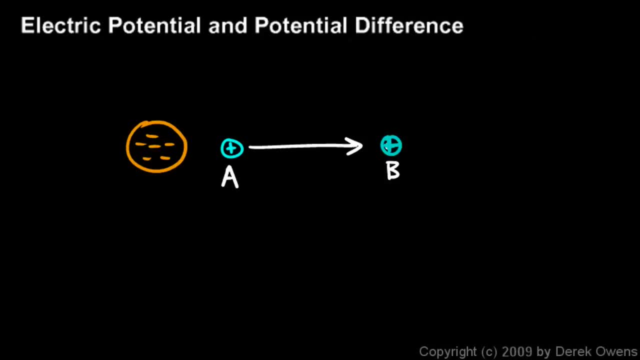 One point represents a point of higher potential energy than the other. Now we can take this analogy one step further. Let's imagine a mass Say here's m- You can think of this as the earth- And here's the gravitational field around the earth. 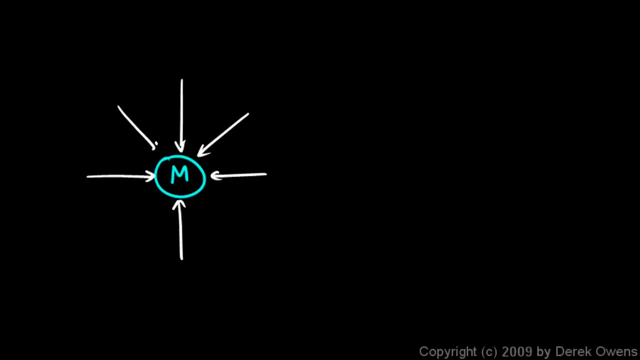 And the gravitational field is directed inward. So things are pulled toward the earth And say here's another little mass m. If we lift this mass up to a point of higher potential energy, it has more potential energy. The work that we've done in lifting it has gone into potential energy. 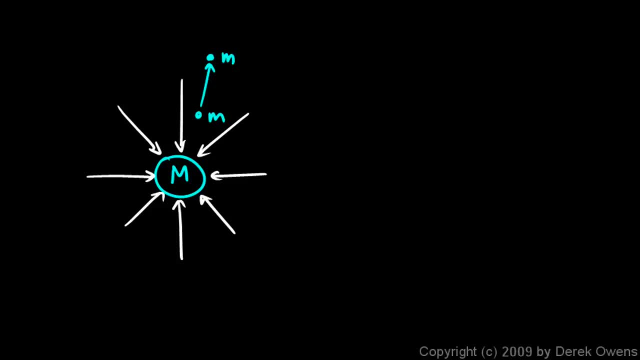 If we then release it, what will happen to the mass? Well, the mass will fall, And when it falls it loses potential energy. And that energy can do two things. It can become kinetic energy. As the mass falls, it picks up speed. 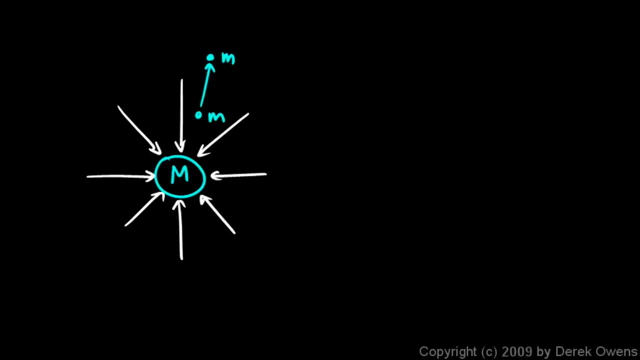 Or the energy can become useful work. Now that first statement, that it can become kinetic energy, that's pretty obvious. We've all seen masses dropped and sure enough, they pick up speed. Things gain speed as they fall. they're gaining kinetic energy. 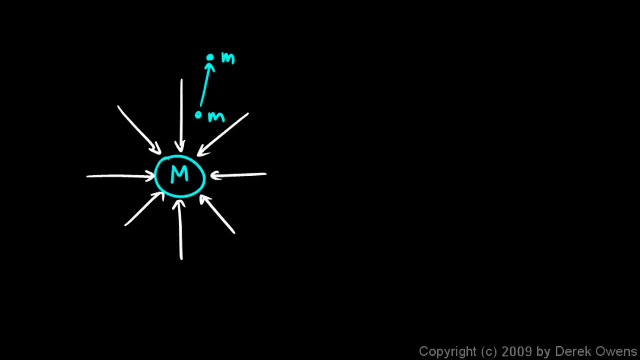 But how about that second idea That the mass falling, when it loses potential energy, that energy can become useful work? That might not be as obvious, So let's look at an example. What's an example of a mass falling and doing useful work? 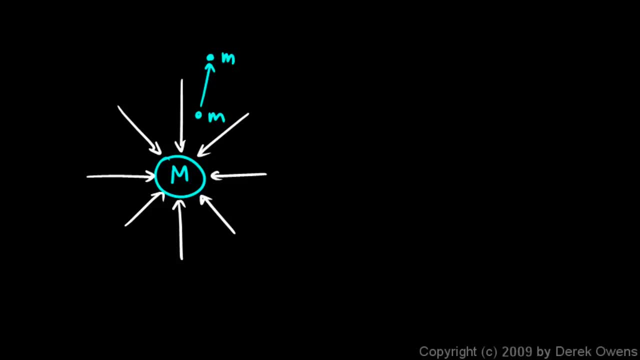 Well, here's a pretty simple example. Imagine a water wheel And you know how a water wheel works. You have a chute of water, A chute of some kind that delivers water up to the top, And the water is caught in these slats here. 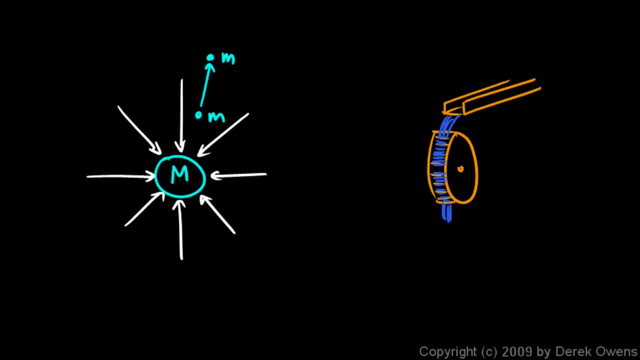 And the weight of the water pushes down on one side of the wheel And it falls out and flows away down here. But that causes the wheel to turn And then the axle of this wheel could be hooked over here to say some stones, some millstones that rotate to grind some grain. 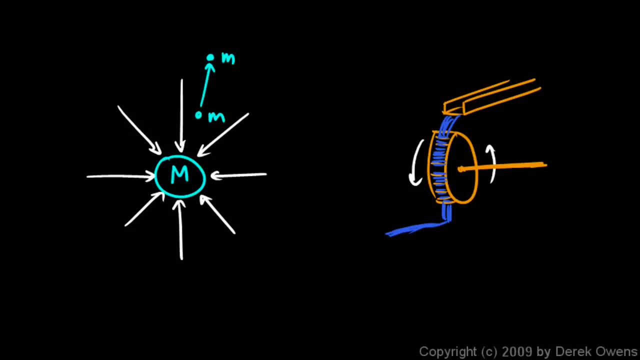 Or it could be hooked into a generator to generate electricity. But the point is, it's the water, the force of the water pushing down. As the water falls, it loses potential energy And it doesn't pick up as much speed as it otherwise would because the water wheel's in the way. 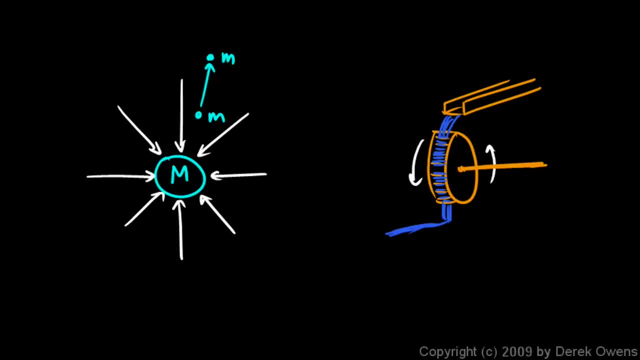 Instead of gaining speed, that potential energy gets converted into useful work as this shaft gets rotated. So that's an example of mass falling in a gravitational field and the potential energy being converted to useful work. The same type of reasoning applies electrically. Let's imagine some charge. we'll call it Q.